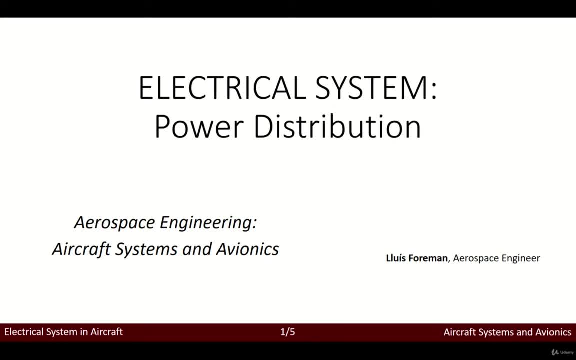 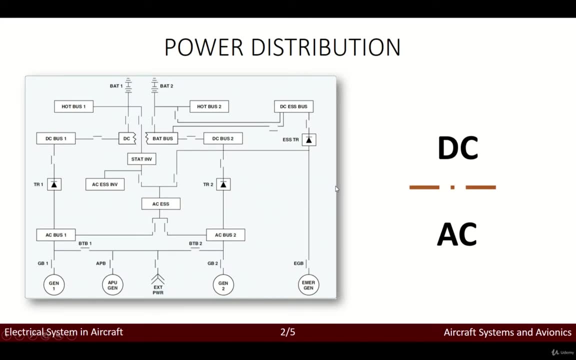 Hey guys, welcome to this new class in the course of Aerospace Engineering, Aircraft Systems and Avionics. Now, today, we will continue to study the electrical system and specifically, we'll be talking about the power distribution Right. so, in terms of the power distribution, again what we see is the schematic that we've seen in other classes. 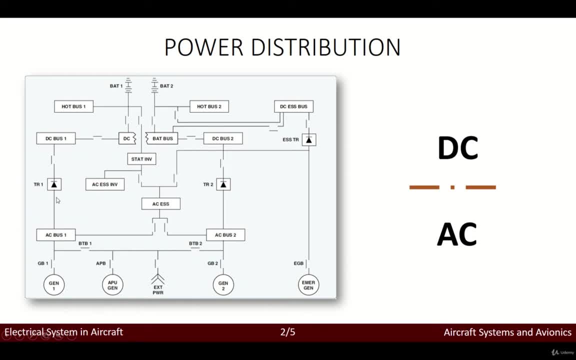 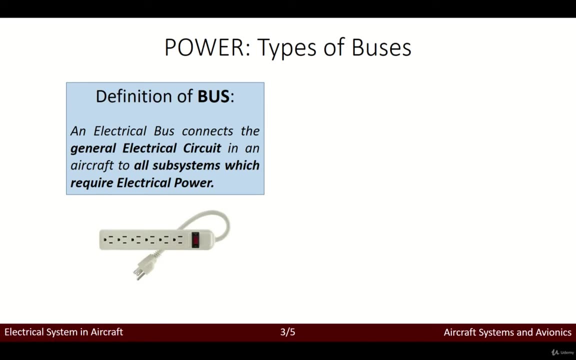 with all the area regarding the alternating current and regarding the direct current, okay, the transformers, the generators and also the different buses for the different users, Right? so the first thing that we need to do now is define what is a bus, Right? so an electrical bus connects the general electrical circuit. 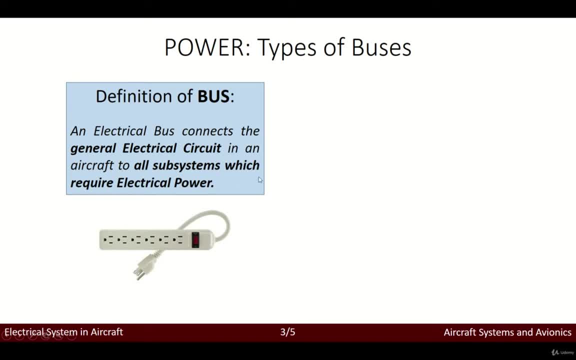 in an aircraft to all the subsystems which require electrical power. So that means you know, any screen, any electrical device on the aircraft needs to be connected through a bus to the main generator system, right to the main electrical system. And this is the you know, the visual concept of a bus. okay, meaning that what we do is connect. 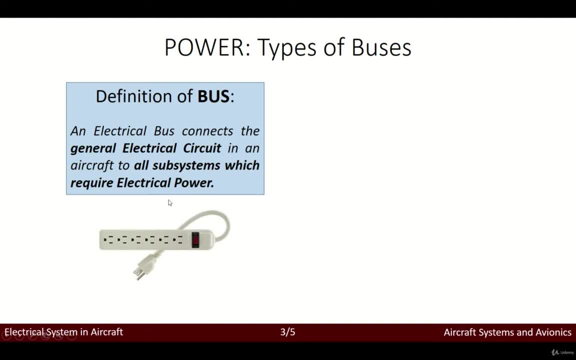 this bus to, you know, to the electrical system, to the generic electrical system, and then we can simply connect all the devices, all the different users that we need, okay, to the bus, right? so this is the idea of the bus, Right? so this is. 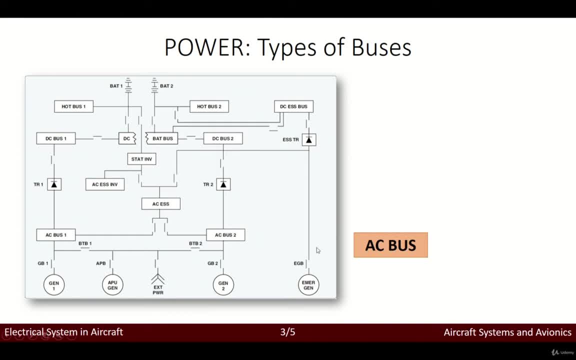 so this is the schematic. again, as we've seen, and just to go quickly through this, we have the alternating current bus. okay, number one, number two, in fact we have the direct current buses over here which are over here, sorry, which is the DC bus one and the DC bus two. 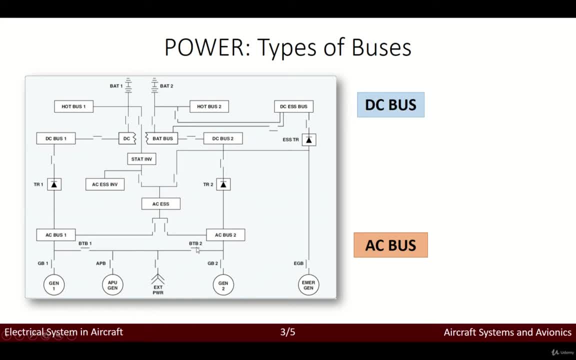 again, remember that we're using the first system and the second system related to generator number one and generator number two on different engines of the aircraft. Then we have the DCESS bus, or what is known as the emergency bus, which is a bus that 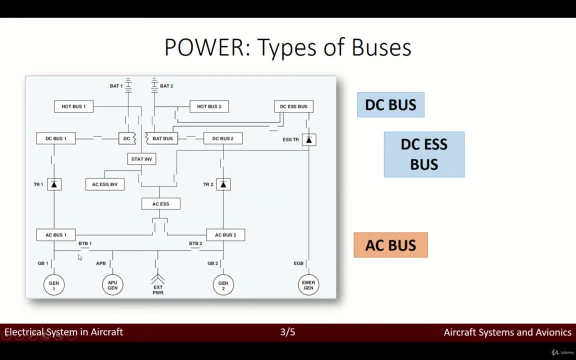 will be used in the case of failure of the generator number one or generator number two. Then we have the alternating current, essential or emergency bus And finally we have the hot buses: hot bus number one and hot bus number two, which the idea of a hot bus is that it always is powered. 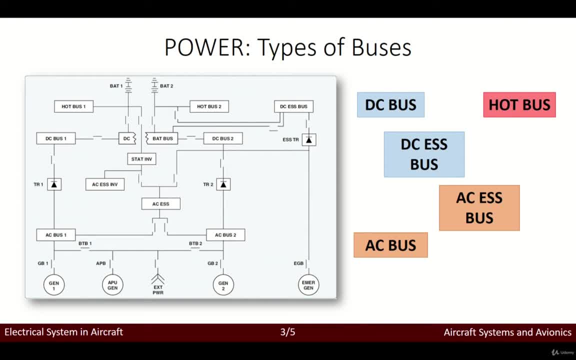 Any energized bus will be hot. any of these buses will be hot at some specific stage. but the common use of a hot bus, the idea of a hot bus, means that it doesn't need a switch to be powered, but rather it simply comes directly from the power source. 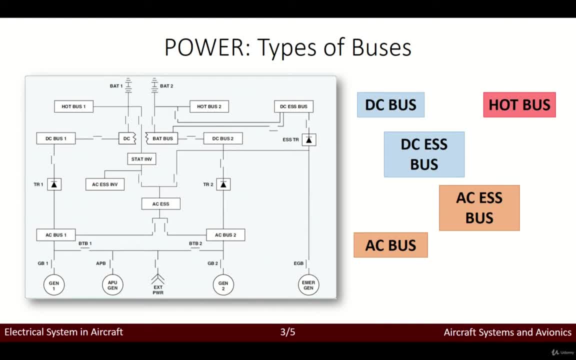 So a hot bus is really a powered bus, but the term is usually described specifically for a bus that can't be powered down. So the hot bus will. The hot bus will always be connected to some kind of supply of energy, and this is extremely. 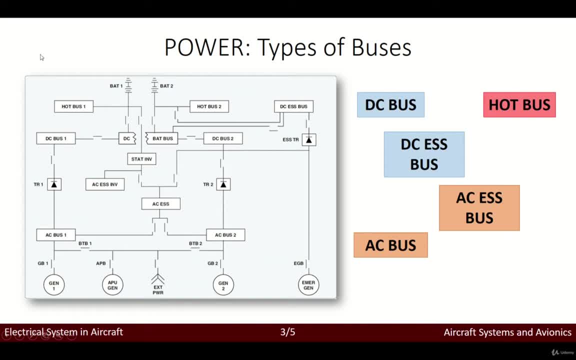 important in the case of aircraft, right. So again, we have just generic, alternating and direct current buses, one and two, depending on the system. We have the essential emergency buses, okay, And finally we have the hot buses. So this is the definition of all the buses right, of all the different connections that 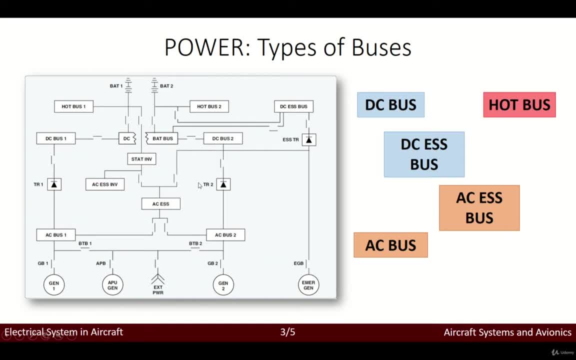 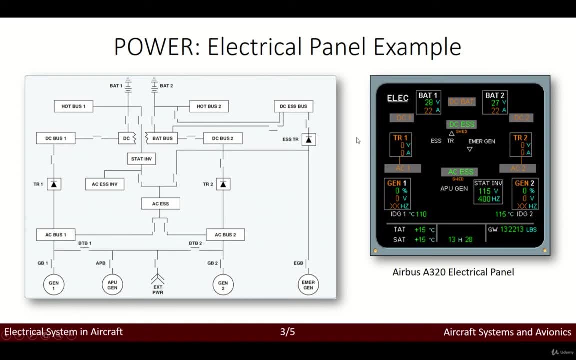 we need in order to get energy- Electrical Electrical energy- to the different subsystems that we need, Right? So this is what you know. if you are a pilot, this is what you will see and this is the way that you can visualize the different systems you know of the electrical power, right? 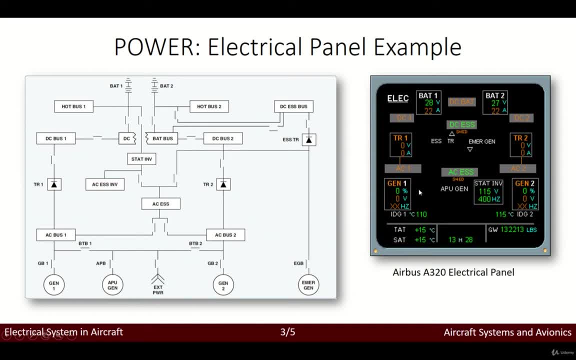 So, for instance, what the generator is doing if it's working, if it's not working, if it's operating okay. You can also see the different buses right: The DC1, DC2, AC1, AC2.. 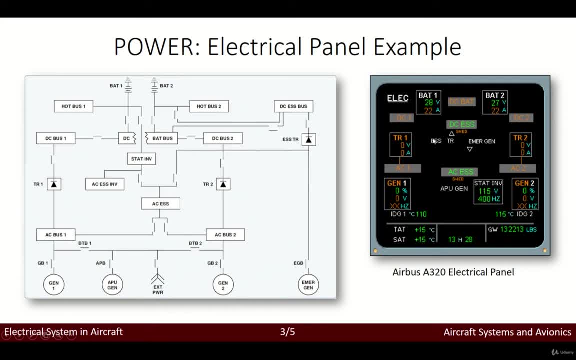 You can also see the different buses right, The DC1,, DC2, AC1, AC2.. With the voltage and intensity, the current of the. you know if it's working, if it's not working, basically. And then you have also the AC emergency and DC emergency buses over here which indicate: 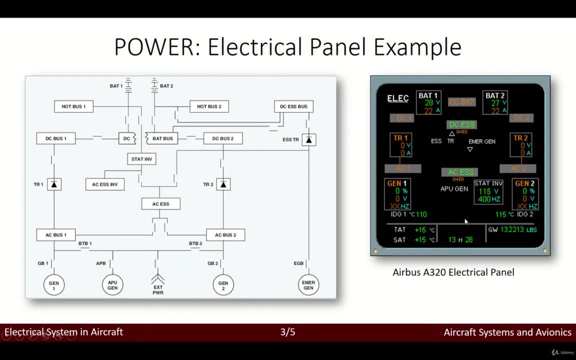 the again, the operation of them. Also, we have the APU generator, which we mentioned before, and, yeah, the batteries and the state of the batteries. okay, So this is, you know, a bit of a summary of all the different systems, how they are operating. 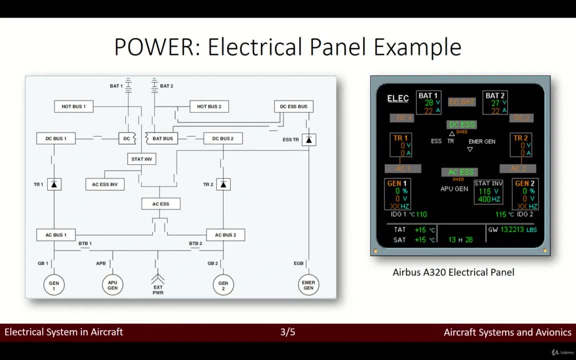 and their current- you know- conditions, okay, So this is what the pilot will see and this is how a pilot is able to identify all the subsystems if you know their operation generally. This is in the case of an Airbus A320, for most aircraft you will see something similar. 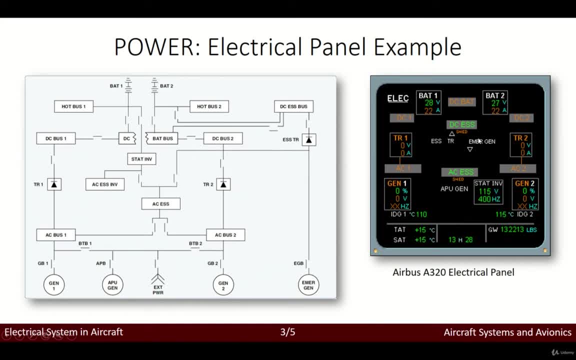 to this. It may vary a bit depending on the aircraft. okay, Right? So yeah, I wanted actually to mention a few more things on here. Okay, So, a bit of the strategy in terms of the alternating currents and the DC currents. 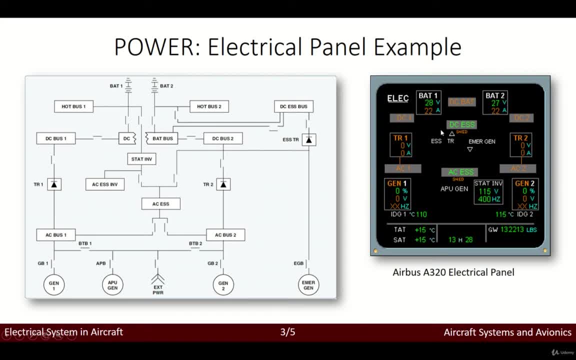 and also the emergency currents. what's the main difference? and so on. Right, So the AC and DC ESS buses provide power to critical instruments, communication and also navigation equipment. okay, So the AC ESS bus is normally powered by the AC bus number one, right? 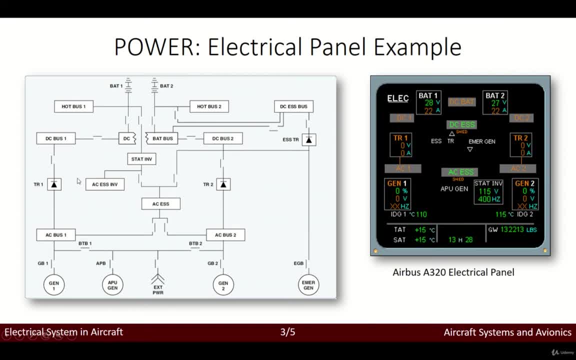 Right, And in case of the AC bus, one failure in case of. you know that this fails. okay, the AC ESS bus can be manually transferred to the AC bus. number two, by selecting the AC ESS feed over here, which is a switch that the pilot can actually alter. okay, on the. 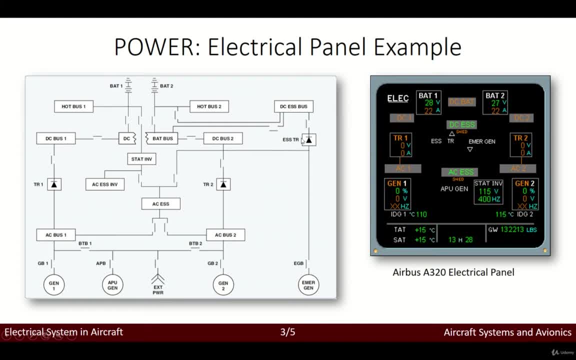 overhead panel, Right. So on aircraft that are modified with the addition of an automatic switching system, which this could be means. just means: okay, Right, So this could be automatic. okay, The switch should not need to be pushed in the case of the failure of the AC bus one. 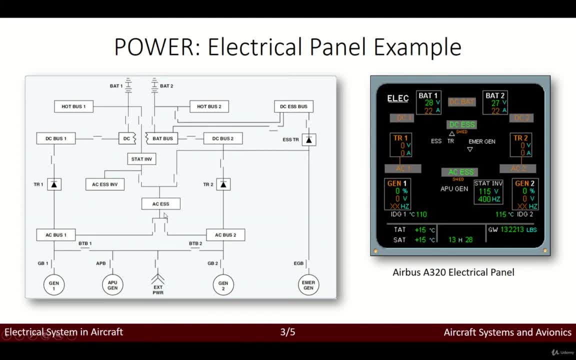 So this is a bit of the strategy used. okay, There's many, many types of different strategies and algorithms that define when an AC ESS bus is working or not. okay, And in the case of the DC ESS bus, it's normally powered by the DC BAT bus. okay. 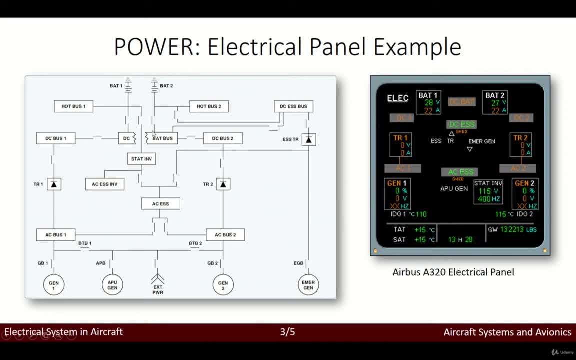 So the battery bus, Right. So this is the battery bus over here. okay, It can also be powered by the ESS TR and also, you know it should be powered. I mean it should be powered by the ESS TR. okay, in the case that the TR one or TR two fail, okay, 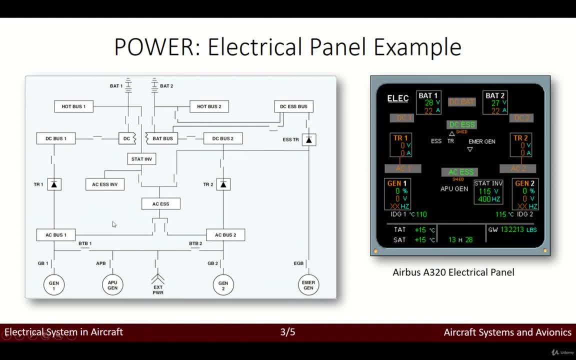 So it basically comes to mean that, depending on the what fails, if there's some failure on the engine, for instance, we of course. if the engine one doesn't work, then we have problems regarding the generator one. We have troubles regarding to powering all the subsystem on this number one area, okay, 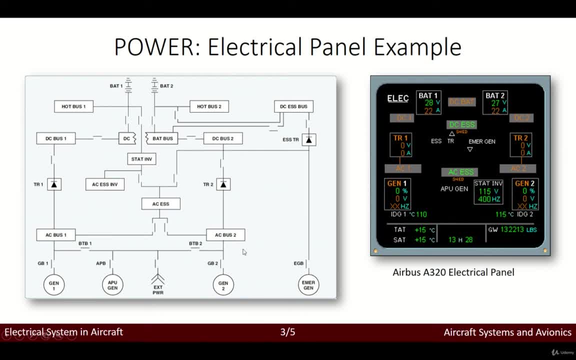 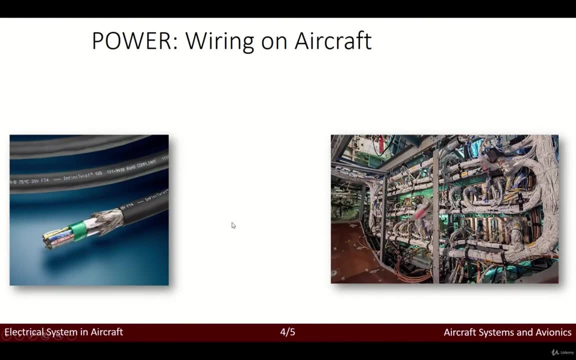 And so we basically need the generator number two to fulfill all the systems. okay, And the way in which this is done. it changes from aircraft to aircraft, but basically you can see that there's always a strategy to make sure that all buses are covered, right? 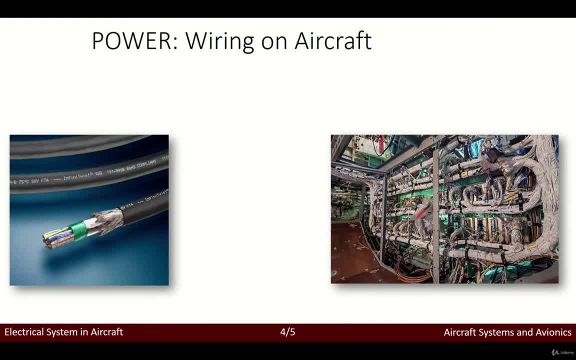 Okay. So again, the most usual, Most general, Okay, Used conductors are copper and aluminum. okay, Each has characteristics that make its use advantage under certain sync up starters right. Also, each has certain disadvantages, okay. So copper has a higher conductivity, for instance, is more ductile, has relatively high tensile. 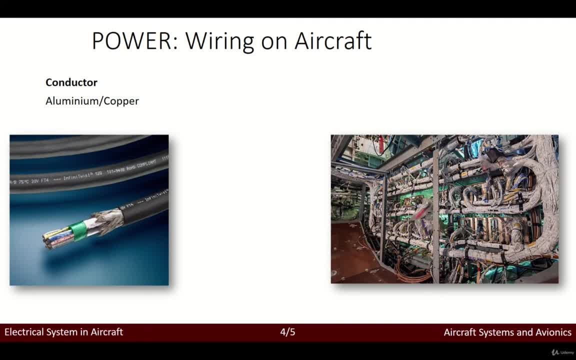 strength and can be easily soldered. okay, Copper is also more expensive and heavier than aluminum, Although aluminum has only 60% of the conductivity of copper. okay, It is used extensively. It's lightness makes possible long spans and it's relatively large diameter for a given. 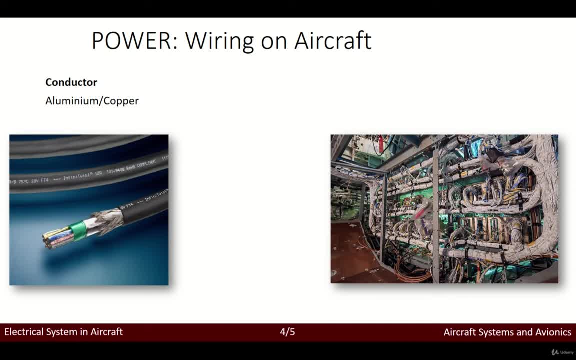 conductivity reduces the corona right. So this is the discharge of electricity from the wire when it has a high potential. Okay, This is a bit technical, but it's actually an advantage. okay, So the discharge is greater when small diameter wire is used. 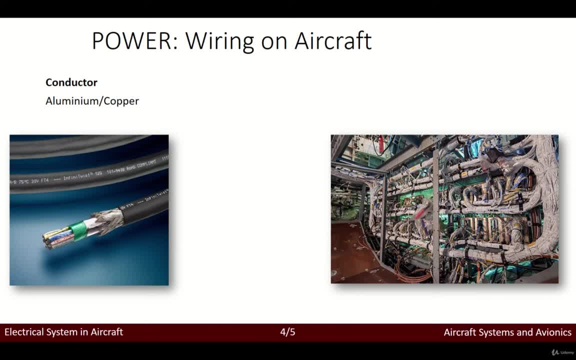 So the discharge is greater when small diameter wire is used. Okay, right then when large diameter wire is used. so it's always a balance on the weight and it's a balance on the amount of conductivity that we have, on the type of conduct. okay, in the case of a design. 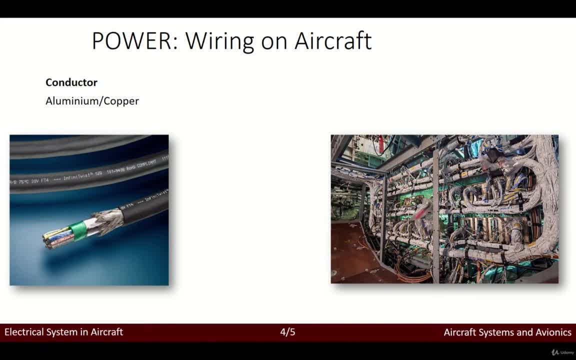 of an aircraft. you just have to take into account them, usually the two possibilities using aluminum or copper, and you should also take into account the- you know, the technological inconvenience that might be related to each one of them. okay, now bare copper develops a surface oxide. okay, coating. 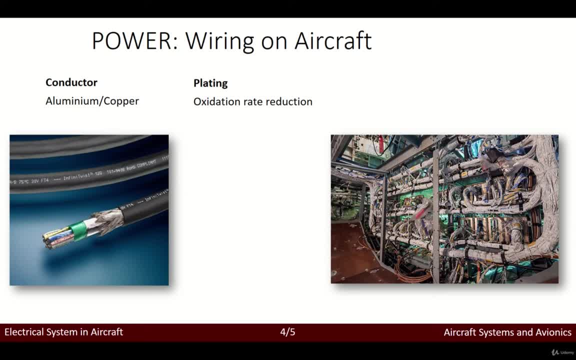 at a rate dependent on the temperature. now, this oxide of film is a poor conductor of electricity and inhibits the term- you know the term: the determination of the wire. therefore, all aircraft wiring has a coating of tin, silver or nickel that has far slower oxidation rates. now, this is essential, okay, in order to make sure that the all the cabling in an aircraft 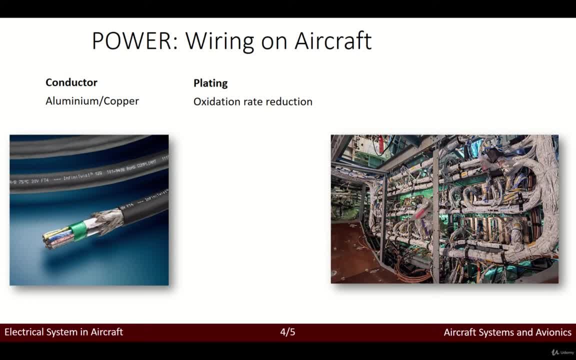 can operate without problem. okay, this is something which is simply needs to be done, right? okay? and in terms of insulation, the type of conducting insulation material varies with the type of installation. characteristics should be chosen based on environment, such as abrasion resistance, arc resistance- okay- corrosion resistance and many more. 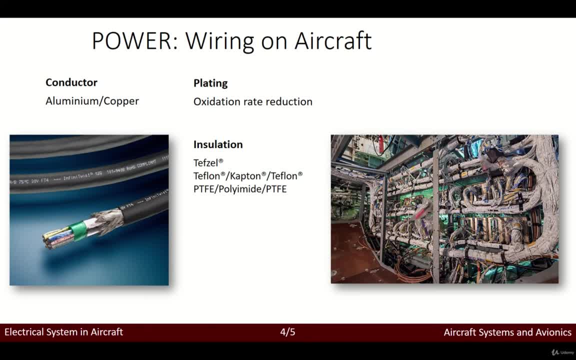 and really such types of insulation materials used commonly. okay, are pvc or captain, for instance, but again, these are not you longer used for new aircraft designs, okay, so mainly what we have nowadays is for new aircraft. okay, we have these technologies which are tfzl, teflon, captain, teflon. 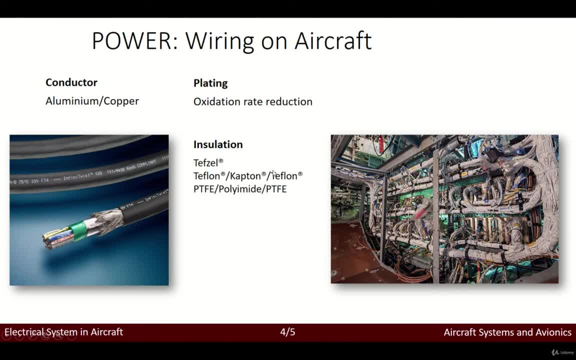 and also the ptfe polymide and ptfe okay. it's a bit more advanced and has, you know, better qualities than most traditional technologies or insulation materials that we had before. right now, with an increase of the number of highly sensitive electronic devices found on modern aircraft, it has become very important to ensure proper shielding for many electric circuits. 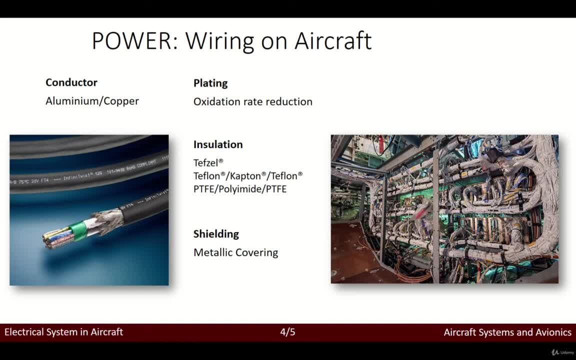 right. so shielding is the process of applying a metallic covering to wiring and equipment to eliminate electromagnetic interference. so basically, what we actually prove, you know, by using a shield, what we're making is the cable, the wiring, electromagnetic free in terms of the electromagnetic, you know, the interference that. 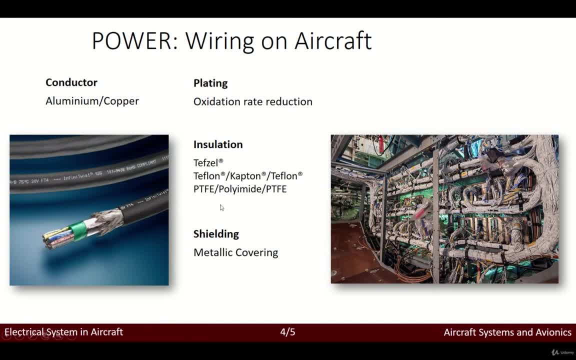 could come from other sources. okay, independent of the cabling. so basically what we're doing is kind of shielding the cables from the surrounding electromagnetic fields. okay, uh, right, so this interference is caused when electromagnetic fields, as i've said before, maybe sometimes also radio waves- induce high frequency voltage in a wire or component. of course this should be you. 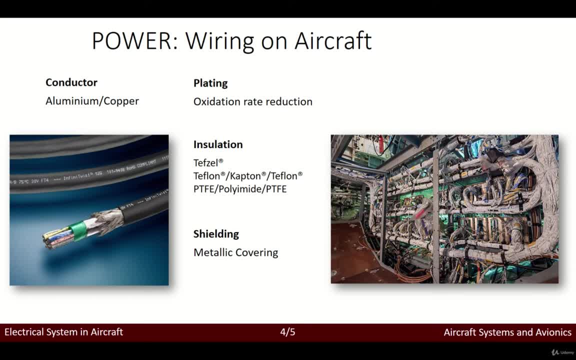 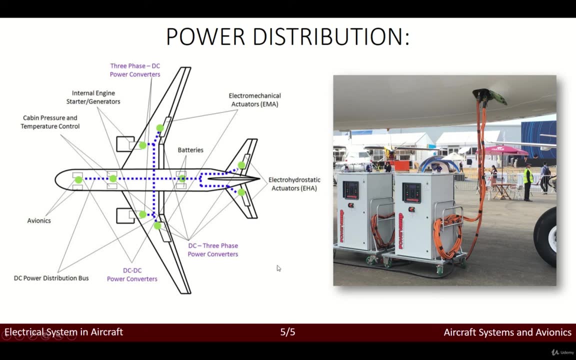 know this would be a problem in our cablings, and the induced voltage can cause system inaccuracies or even failure. okay, so basically we also need shielding for all of our wiring on aircraft, right? so what else? yeah, this is a bit of an schematic of the electrical system, okay.